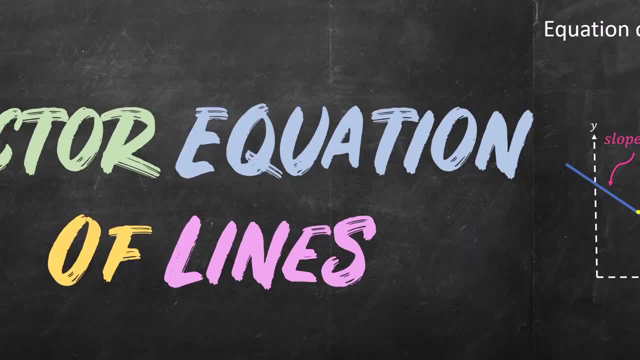 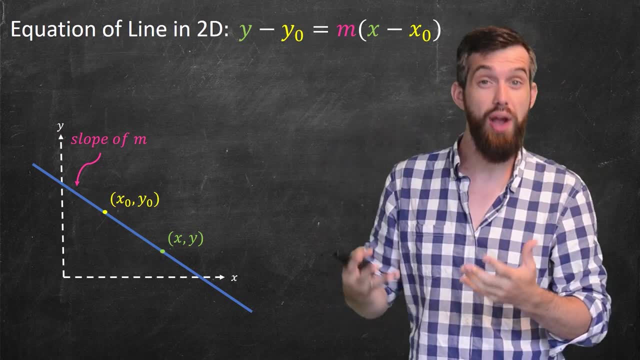 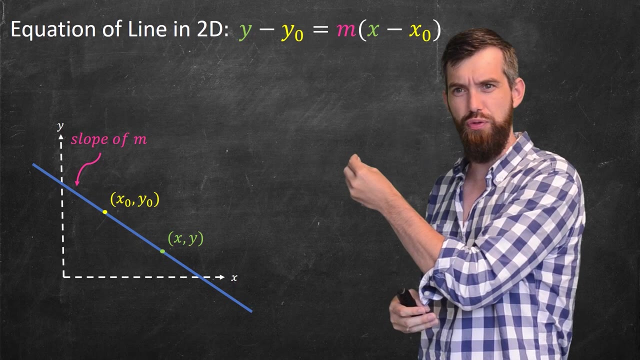 In single-variable calculus we've studied the equation of a line In its point-slope format. it would be y minus y-naught. is m the slope, x minus x-naught? The x-naught- y-naught sort of fixes a location where the line has to go through it. but there's many lines that go through any. 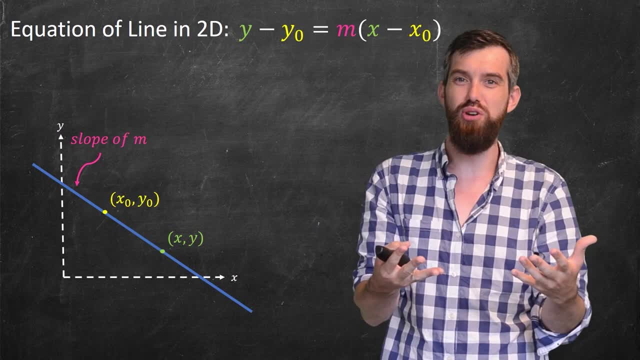 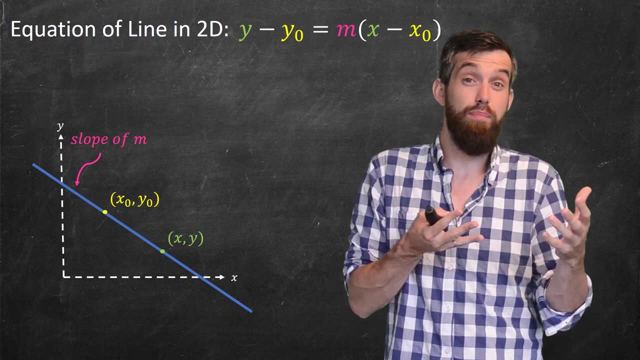 particular fixed point. So I also have to give you something about its sort of orientation or how it tilts in the plane, and that's what's given by the slope m, And then, if I have some other point, a point x, y, that it needs to satisfy this particular condition. So now what? 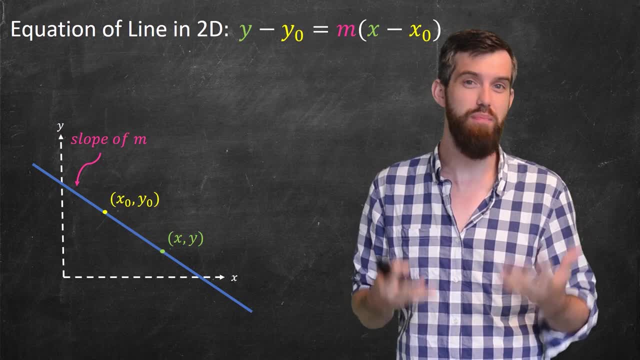 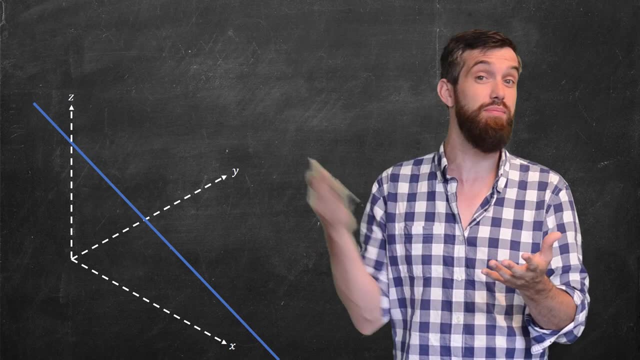 we want to do in this video is generalize this to higher numbers of dimensions. So let's consider the three-dimensional case. I've got an x, y and z-axis and I've got some line that goes through this particular space. Now what I'm going to do to find an equation of this line is rather analogous. 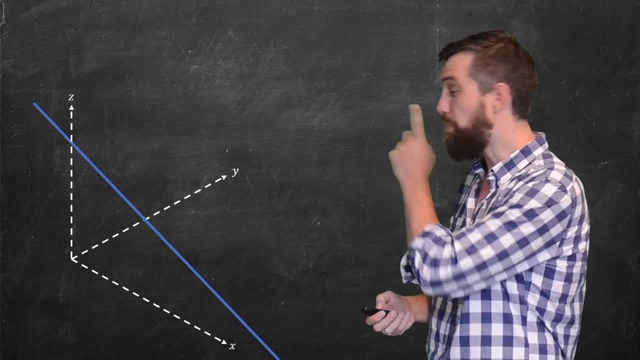 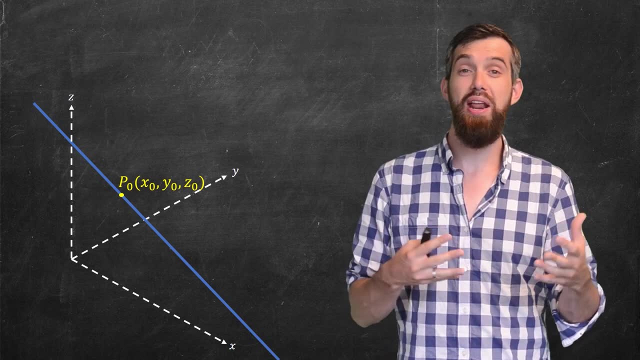 to the lower-dimensional case. First of all, I'm going to put some particular point on that line, some p-naught that has coordinates x-naught, y-naught and z-naught, And while I'm at it, I'm going to define a vector: r-naught, And r-naught is 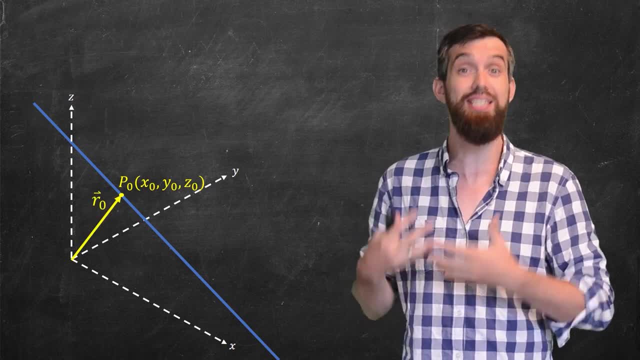 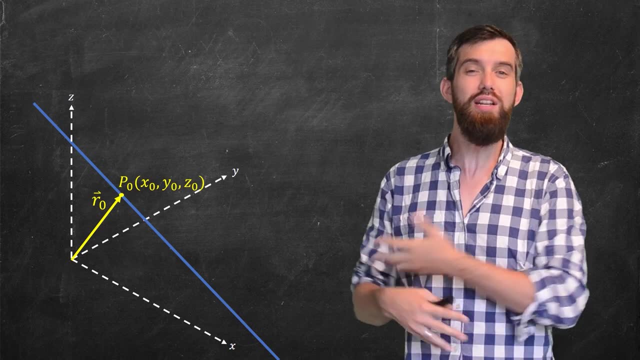 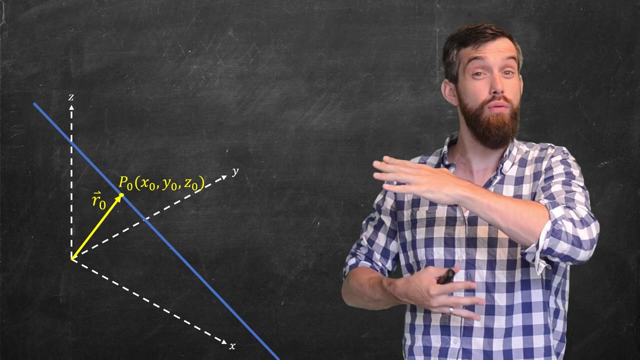 the vector that begins at the origin, that's its tail, and its tip is at this point p-naught. This fixed point is analogous to the x-naught, y-naught we saw before. But what's the analogy for the slope, the m, the way that that line tilts or orients itself in now three dimensions? 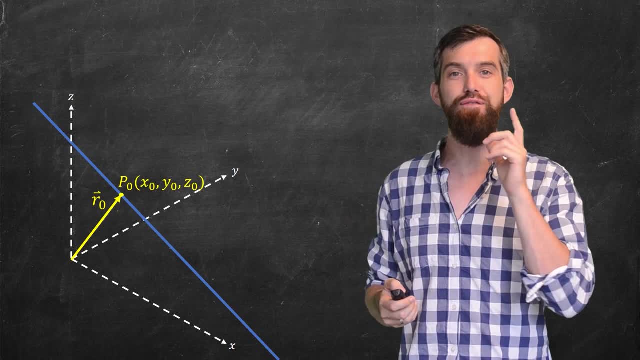 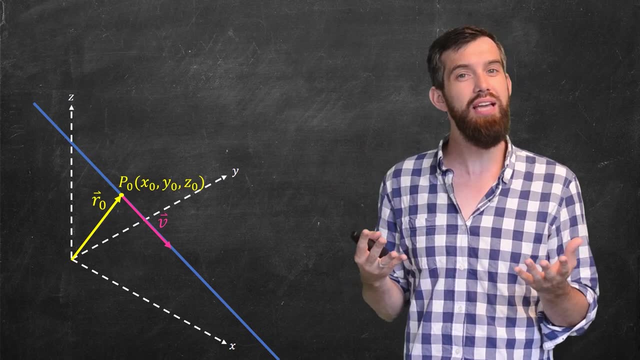 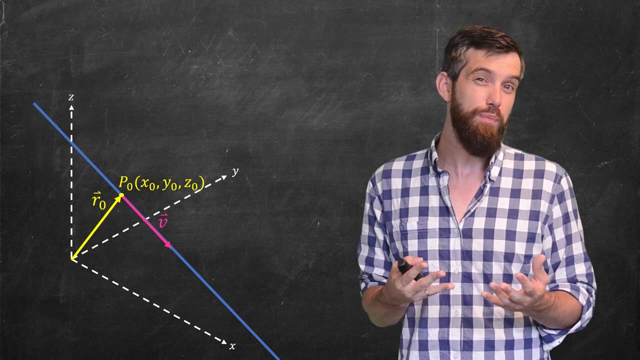 Well, instead of just a single scalar, I'm going to give you a vector. It is the vector v, and v is just some vector, some non-zero vector that lies along the line, That is. this vector v is completely parallel to the line. Now, the hope is this is going to be sufficient. 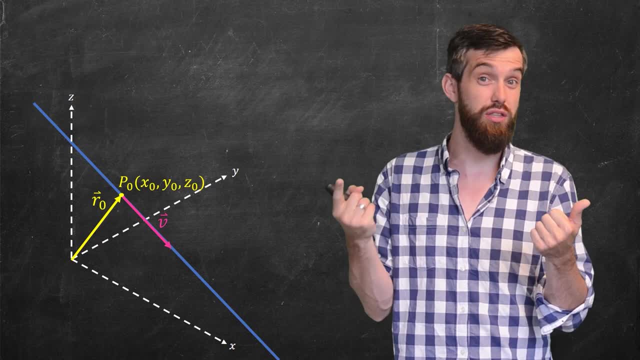 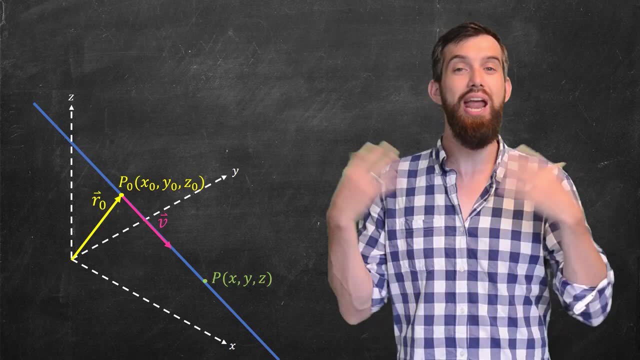 Knowing this point and knowing this v sort of analogous to the slope before, is enough to describe all the points on this line, That is, if I take some other point, let's call my generic point p. it's got coordinates x, y, z. these are completely generic. and while I'm at it, 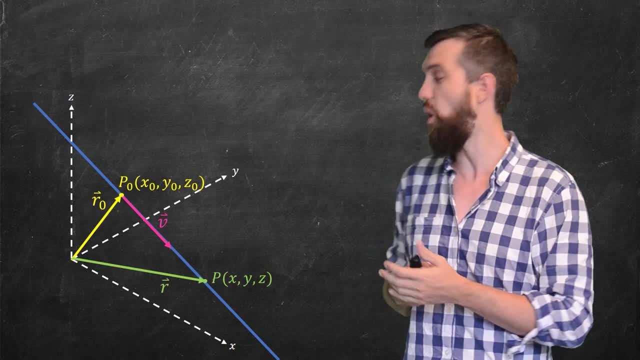 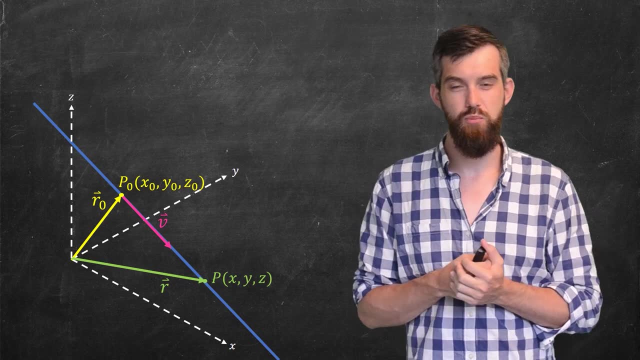 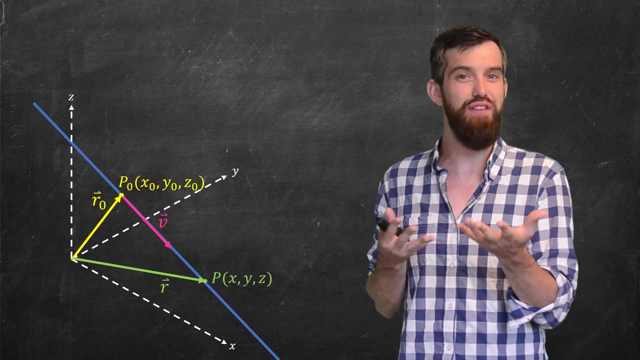 I'll call the vector that goes from the origin out to this p. I'll call that thing r, And what I want to do is find some constraints on these x, y and z. Now you'll notice that I'm getting close to a triangle here. I have this r-naught vector and I can add the v vector, but the tip of 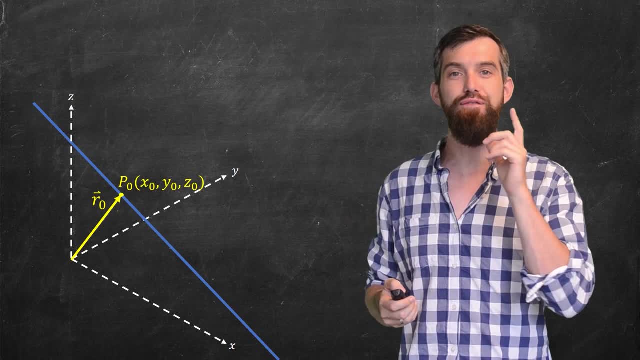 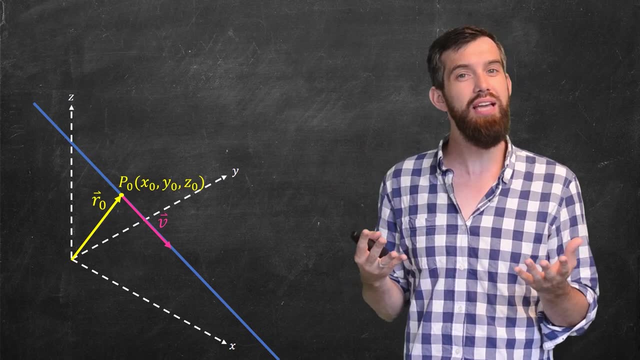 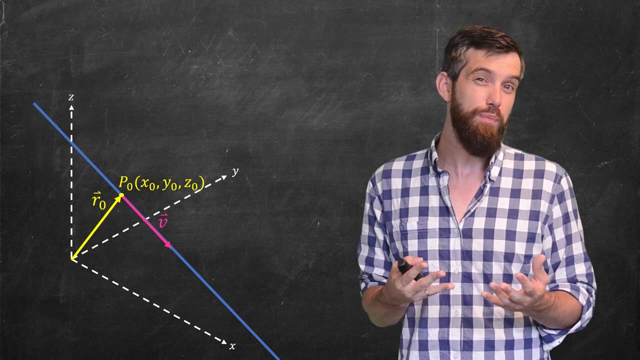 Well, instead of just a single scalar, I'm going to give you a vector. It is the vector v, and v is just some vector, some non-zero vector that lies along the line, That is. this vector v is completely parallel to the line. Now, the hope is this is going to be sufficient. 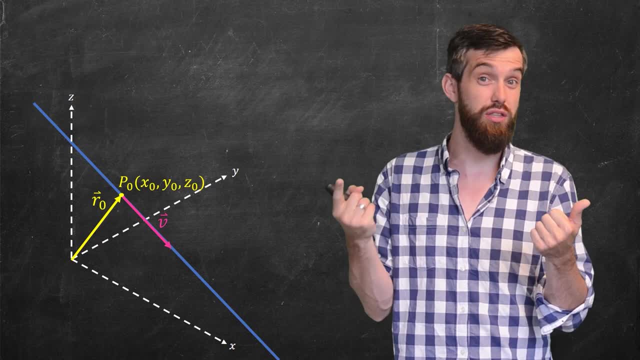 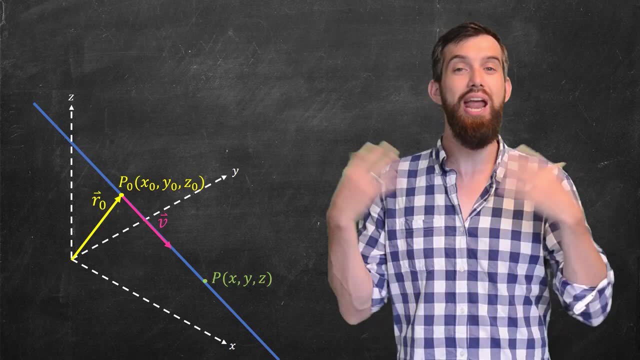 Knowing this point and knowing this v sort of analogous to the slope before, is enough to describe all the points on this line, That is, if I take some other point, let's call my generic point p. it's got coordinates x, y, z. these are completely generic. and while I'm at it, 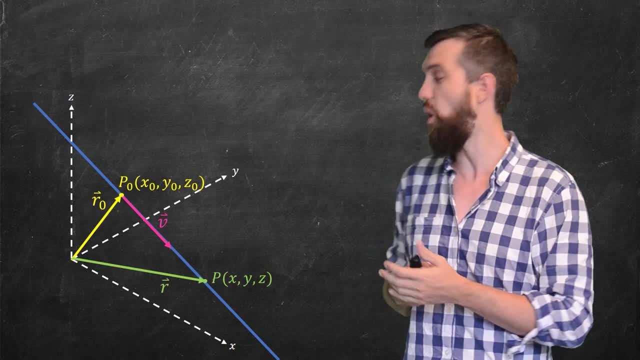 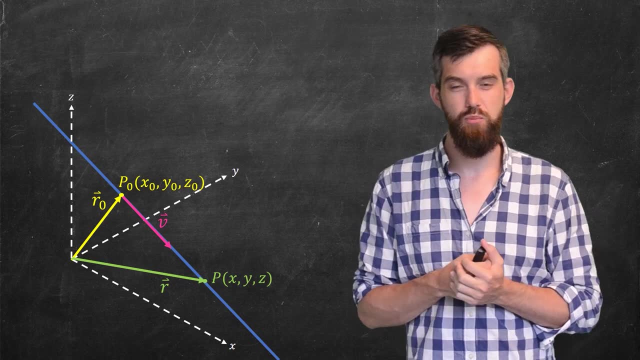 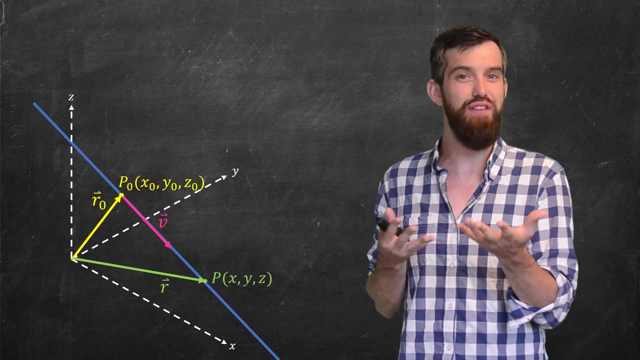 I'll call the vector that goes from the origin out to this p. I'll call that thing r, And what I want to do is find some constraints on these x, y and z. Now you'll notice that I'm getting close to a triangle here. I have this r-naught vector and I can add the v vector, but the tip of 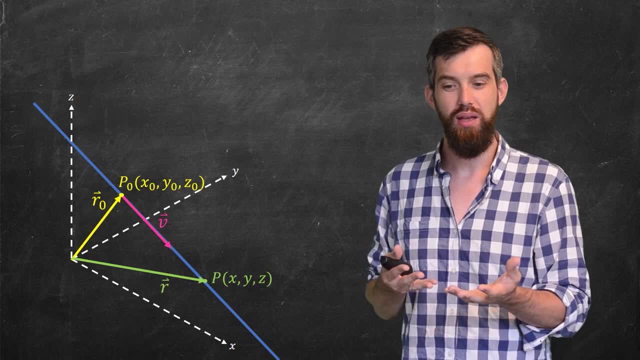 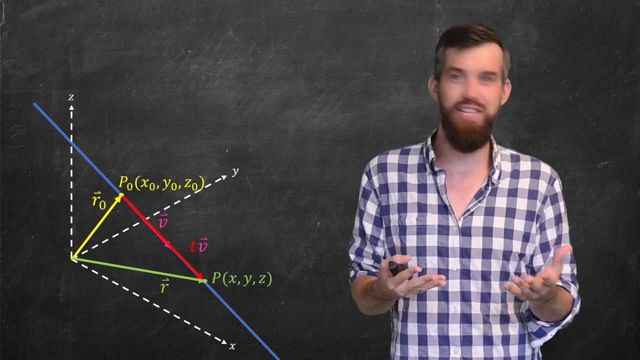 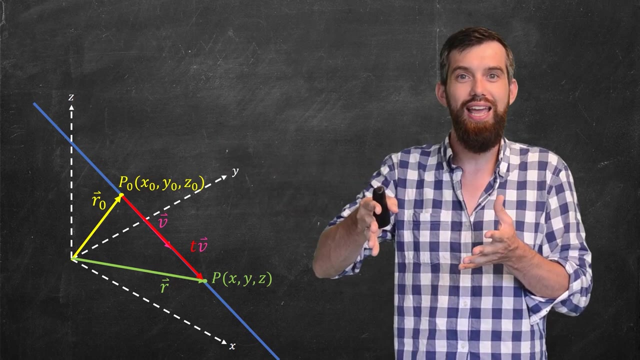 that is not actually at the point p. But what if I stretched out that v vector a little bit? What if t is just some scalar and the idea is I've taken the vector that is on the line and I've stretched it out until its tip is just going to be at this point p? Well then I really do have. 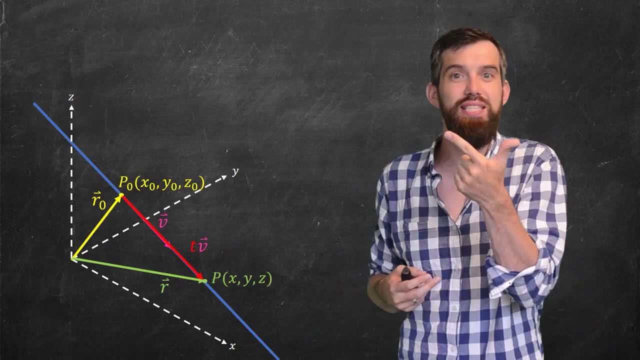 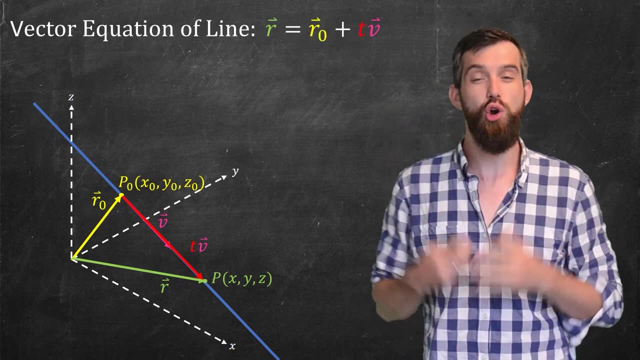 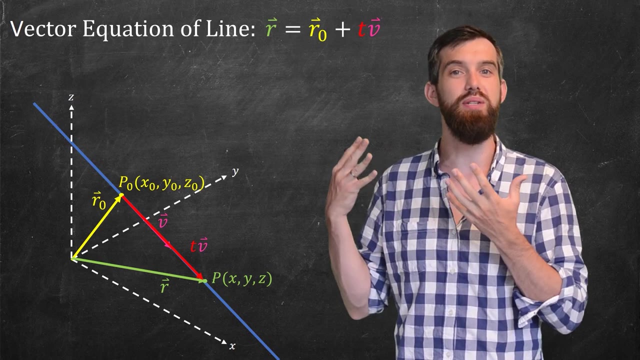 a triangle and I can say that the r-naught plus this t v is going to be equal to the r vector, That is, writing it in its vector format. I can say that the equation of the line of three dimensions is going to be that the r vector can be written as the r-naught plus a scalar multiple. 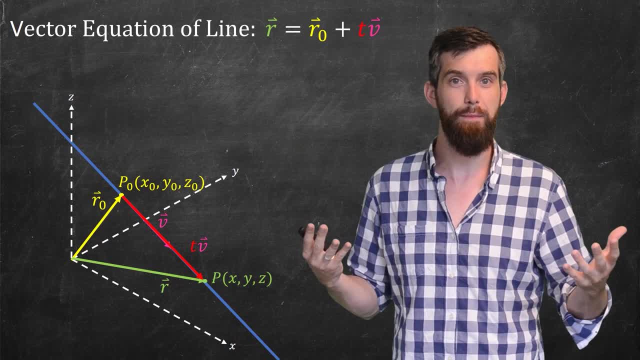 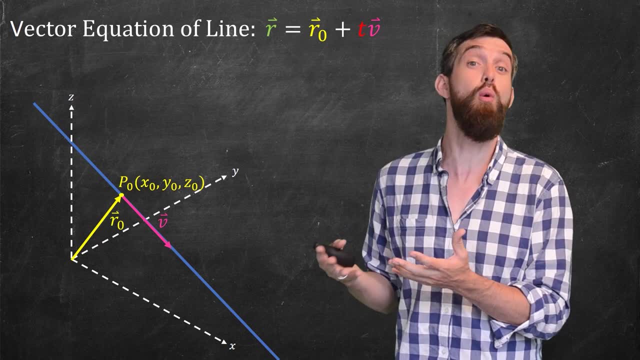 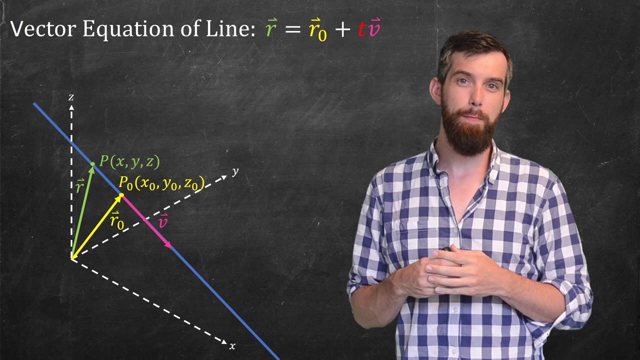 of that v vector, And that's my equation of a line. Now, the idea of this construction is that it works, no matter where that p is, where the point x, y, z is, For instance, if I take this other p and this other r, that goes out to it. well, now I can still make a triangle. 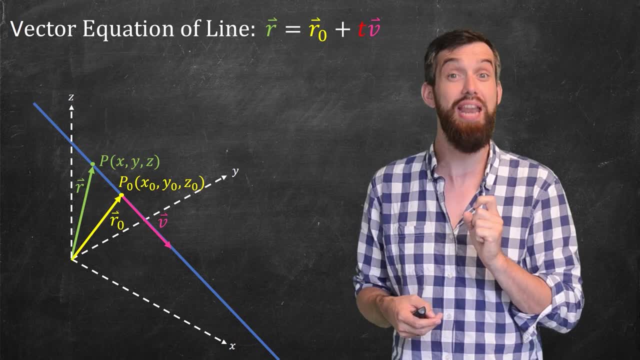 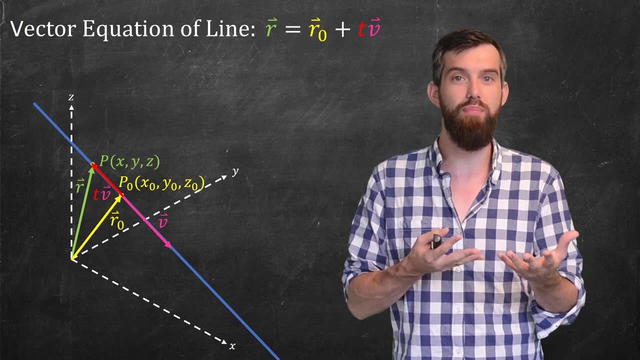 but that t is going to have to be a negative value now, and probably a negative less than one, But I can still make a triangle by doing that. I can say that my new r is the o? r-naught plus this new t times v. So when I think of this, I think I've got one fixed point. 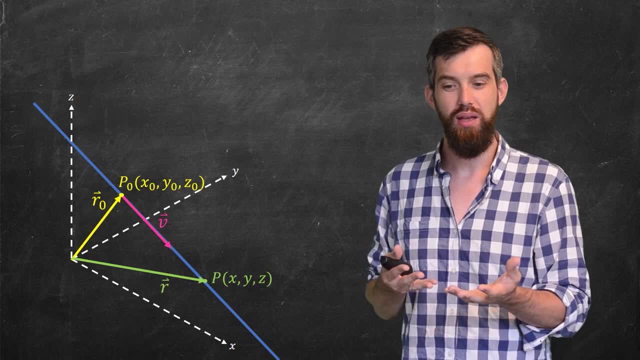 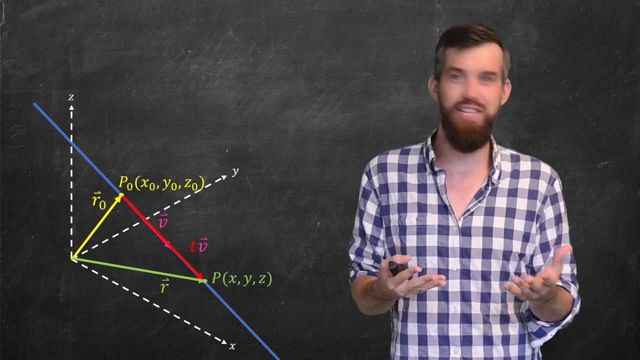 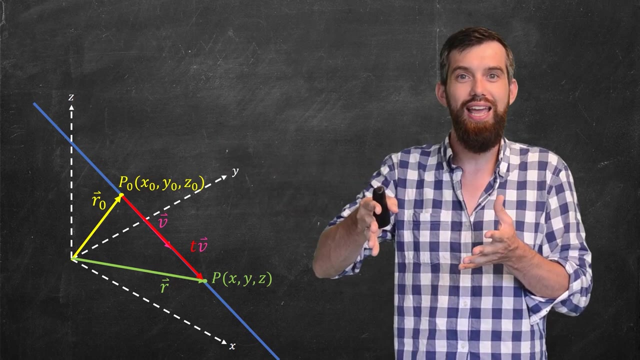 that is not actually at the point p. But what if I stretched out that v vector a little bit? What if t is just some scalar and the idea is I've taken the vector that is on the line and I've stretched it out until its tip is just going to be at this point p? Well then I really do have. 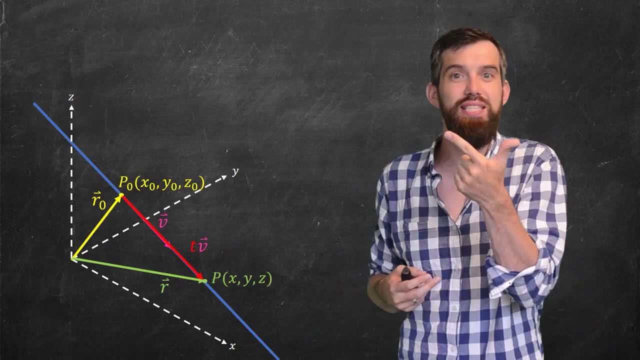 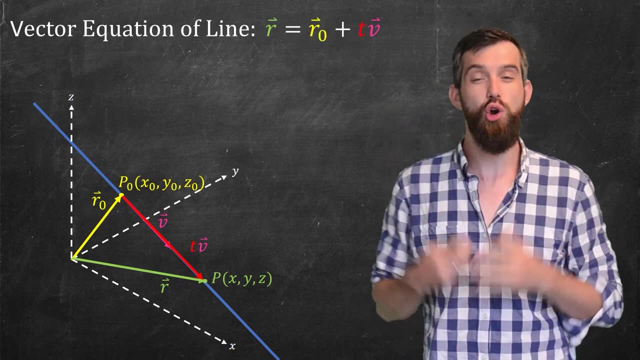 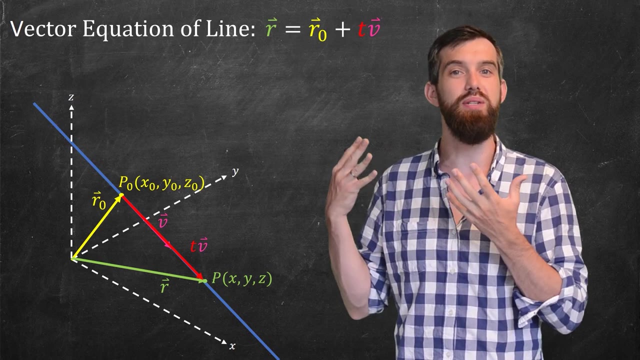 a triangle and I can say that the r-naught plus this t v is going to be equal to the r vector, That is, writing it in its vector format. I can say that the equation of the line of three dimensions is going to be that the r vector can be written as the r-naught plus a scalar multiple. 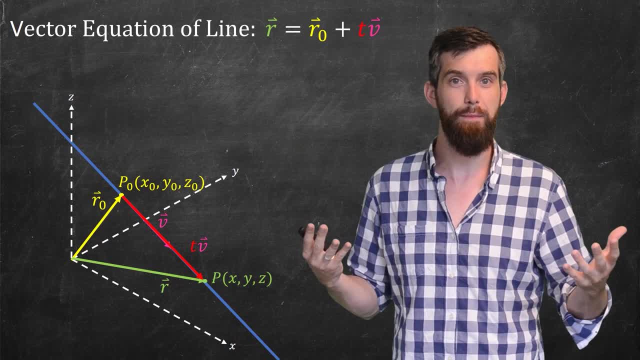 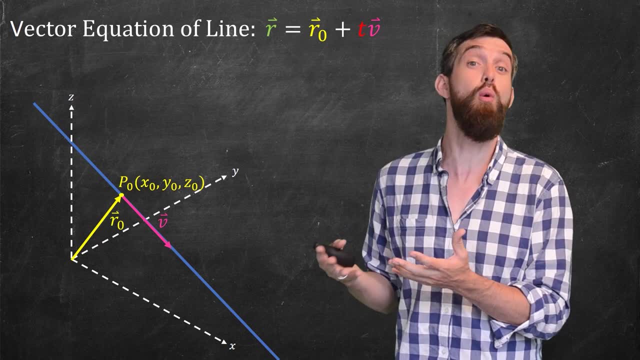 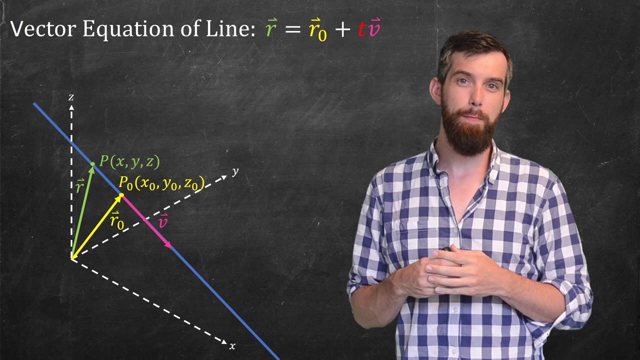 of that v vector, And that's my equation of a line. Now, the idea of this construction is that it works, no matter where that p is, where the point x, y, z is, For instance, if I take this other p and this other r, that goes out to it. well, now I can still make a triangle. 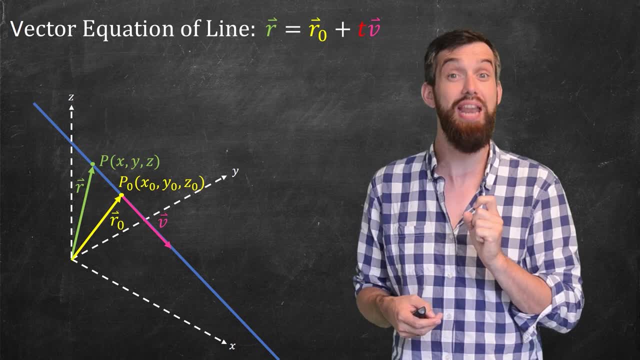 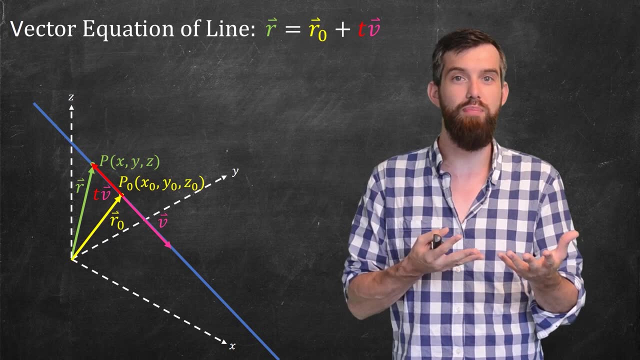 but that t is going to have to be a negative value now, and probably a negative less than one, But I can still make a triangle by doing that. I can say that my new r is the r-naught, plus this new t times v. So when I think of this, I think I've got. 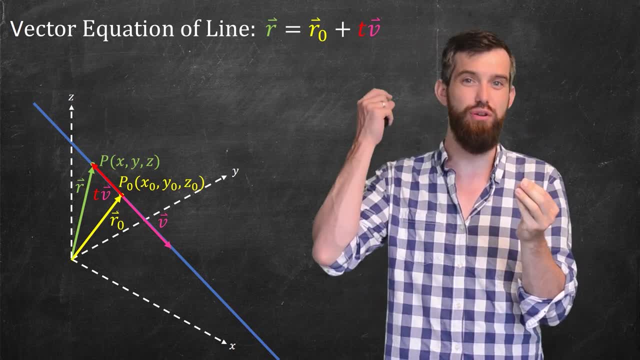 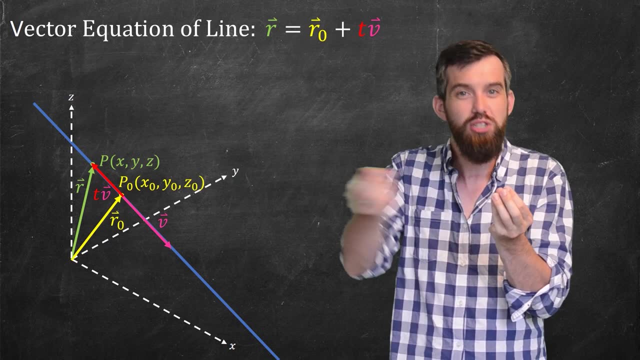 one fixed point, this x-naught, y-naught, z-naught. I have this sort of direction vector along the line of the v And by starting at the p-naught and going out some multiple of that direction vector I can get anywhere else on the line. 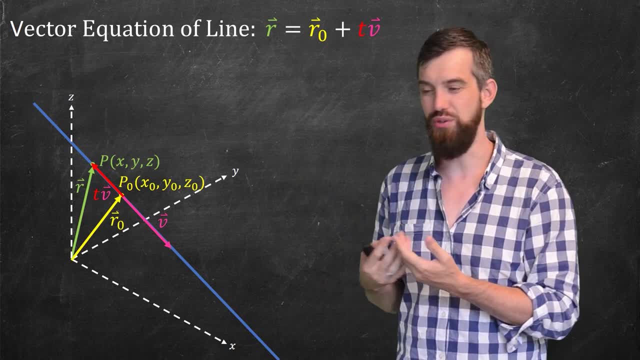 To think about this sort of analogously with driving down a highway. if you say you want to go some distance down the highway, you actually have to do two things. First of all, you have to get on the highway, Like you go from your origin to where you'll be after you're above. First of all, 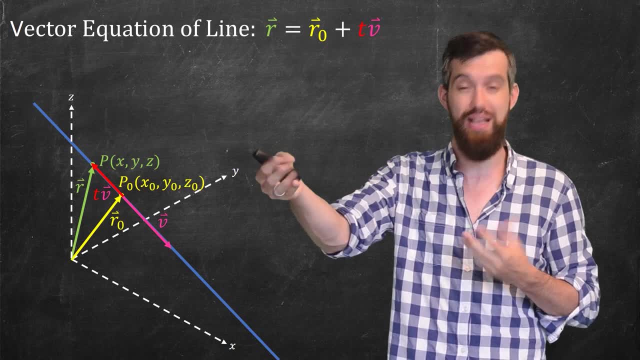 you have to get on the highway, like you go from your origin to where you're at, Like you have to go to corruptions, which is indicated by arrows. You actually have to hurt outside. So I find out the now You go from your origin to the first location on the highway. that's kind of like your p-naught. 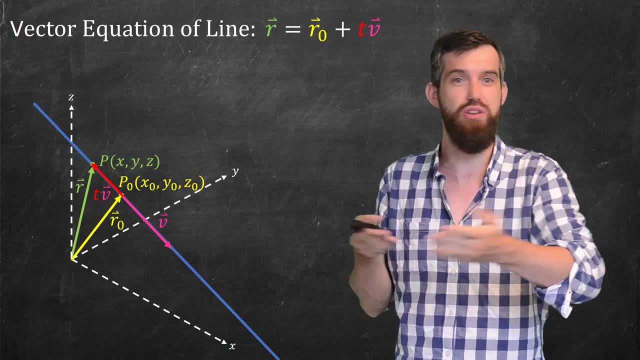 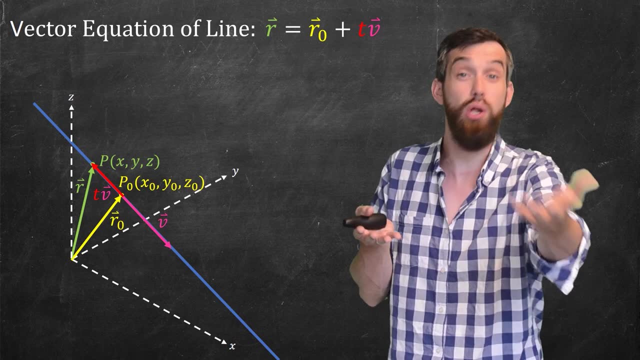 And then you drive down the highway. well, you may be specifying- are you going north or are you going south, but you have your direction, your v-vector, and then you do some multiple of that. Maybe you're going to go, say, 100 kilometers down this particular highway. 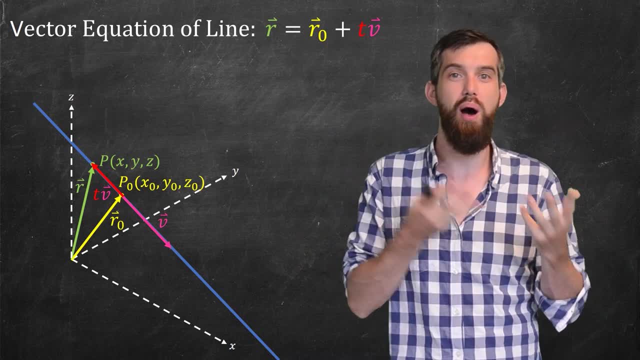 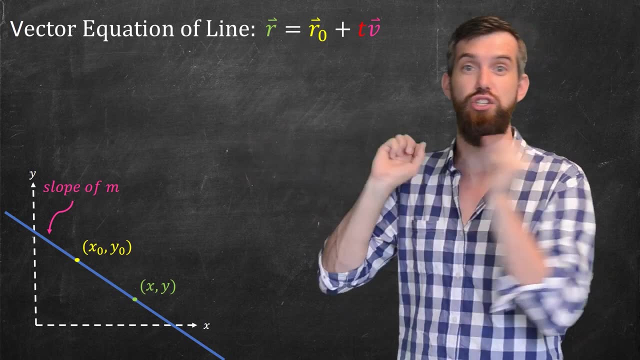 So in that same analogy we can say that our r is equal to an r-naught plus a t-v. Now you might be thinking that these two different equations- the vector equation that works generally in n dimensions, and the one we saw before that works in the plane- 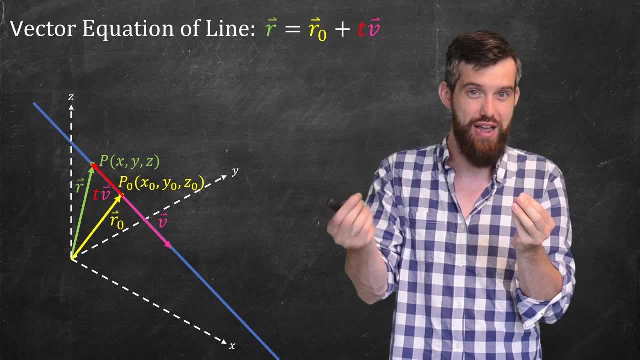 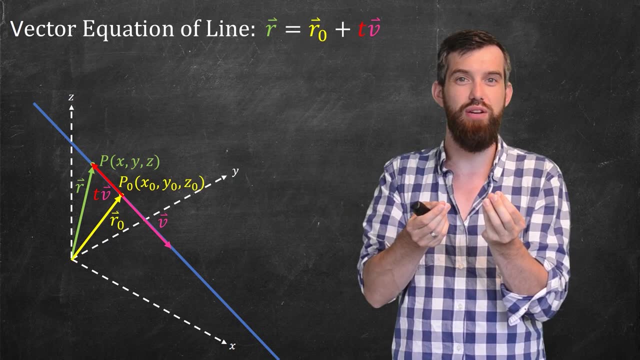 this x-naught, y-naught, z-naught. I have this sort of direction vector along the line of the v and by starting at the p-naught and going out some multiple of that direction vector I can get anywhere else on the line. To think about this sort of analogously with driving. 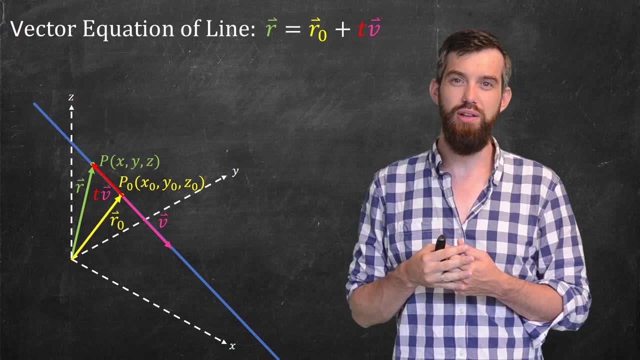 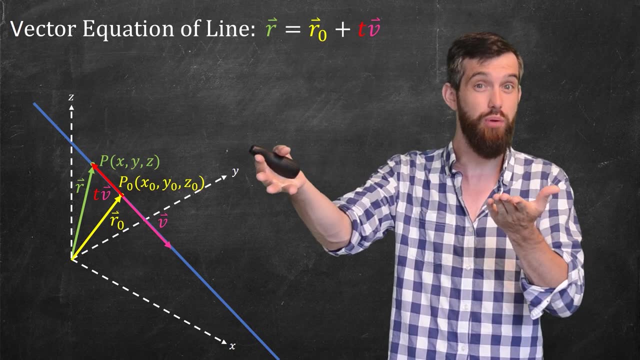 down a highway. if you say you want to go some distance down the highway, you actually have to do two things. First of all, you have to get on the highway, like you go from your origin to the first location on the highway, that's kind of like your p-naught- And then you drive. 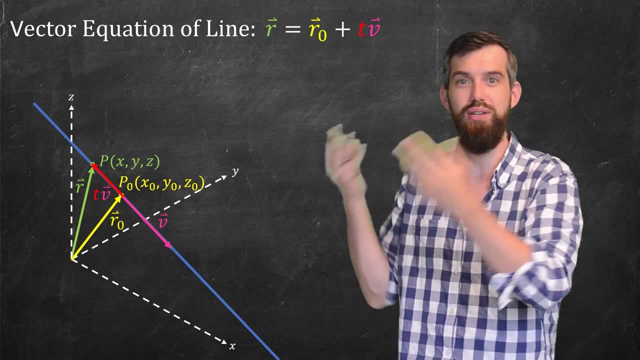 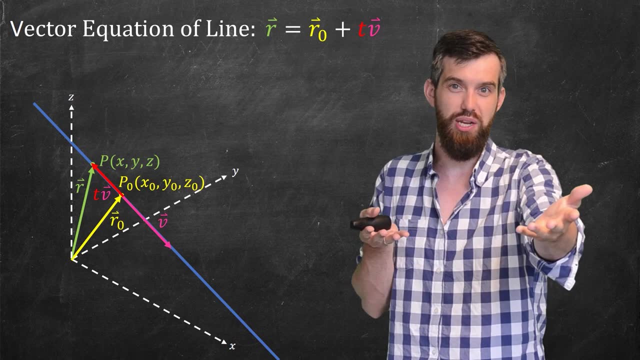 down the highway. well, you may be specifying you're going north or you're going south, but you have your direction, your v vector, and then you do some multiple of that. Maybe you're going to go, say, 100 kilometers down this particular highway. So in that same analogy, we can say that: 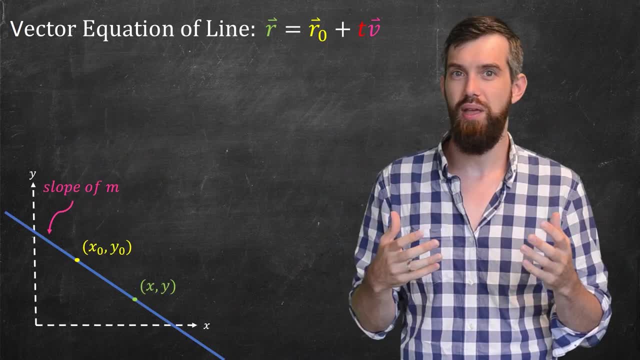 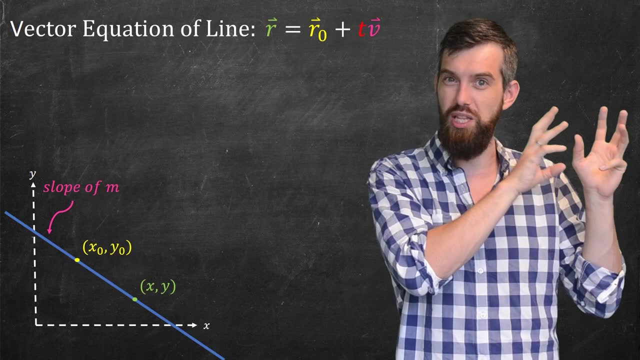 our r is equal to an r-naught plus a t v. Now you might be thinking that these two different equations- the vector equation that works generally in n dimensions and the one we saw before that works in the plane- actually look pretty different. There's a t in this vector equation. 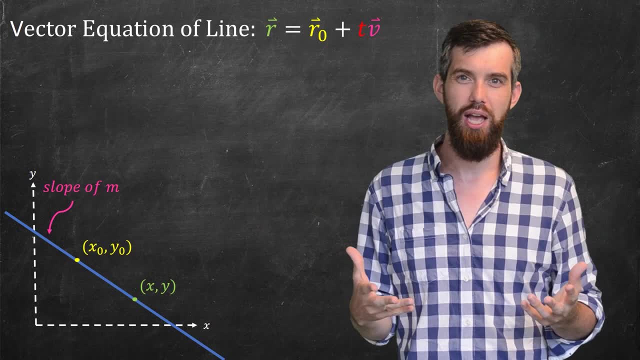 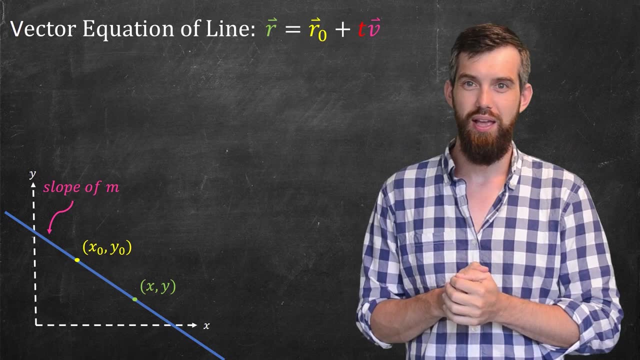 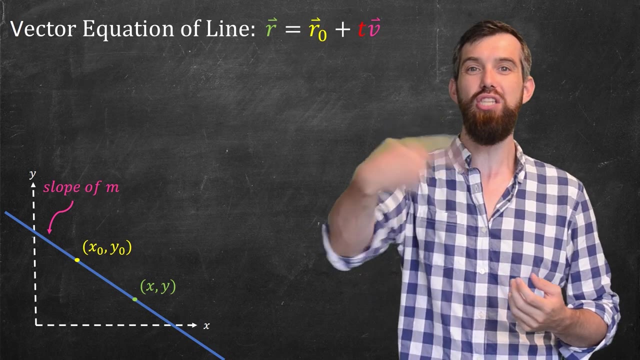 for example, but not prior. So what's going on there? Well, if I imagine this vector equation applying in the two-dimensional case, what would be the v vector? Now, if I chose, for instance, to step one to the right? well, what would happen? Because I have a slope m for my line. 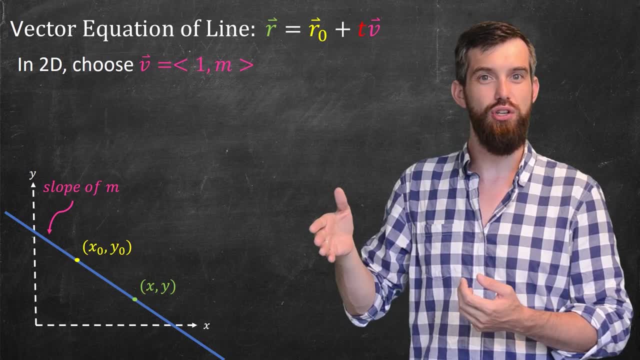 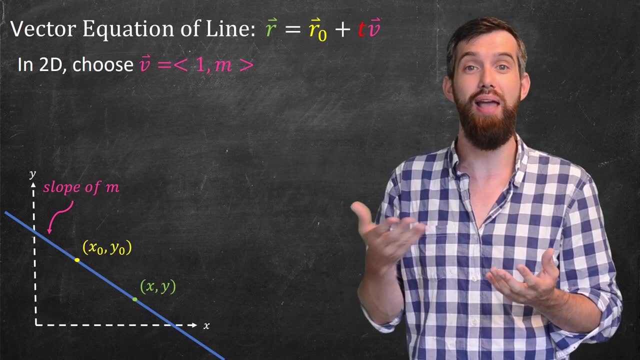 if I'm going to step one to the right, then I'm going to go up the amount m, Which is to say that my v vector, in two dimensions, could be written as one comma m. So then if I use that and I take this vector equation, which, in two dimensions, would really be separated into, 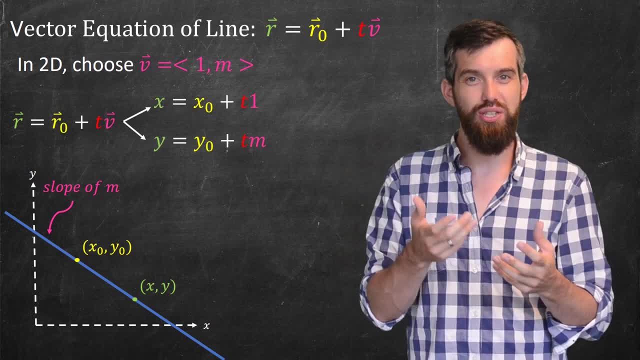 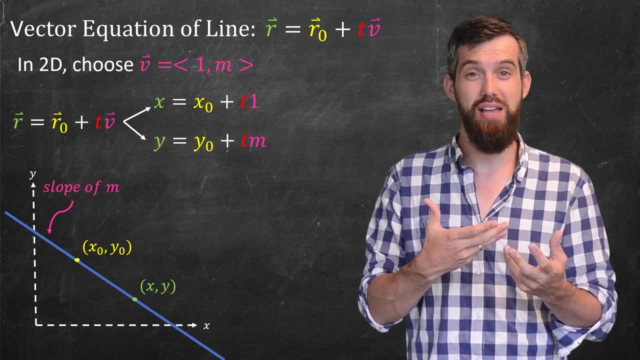 two different equations. so I'd have: x is equal to x-naught plus t times one, and y is equal to y-naught plus t times m. then if I solve for t and plug it in, I get exactly what we had before. 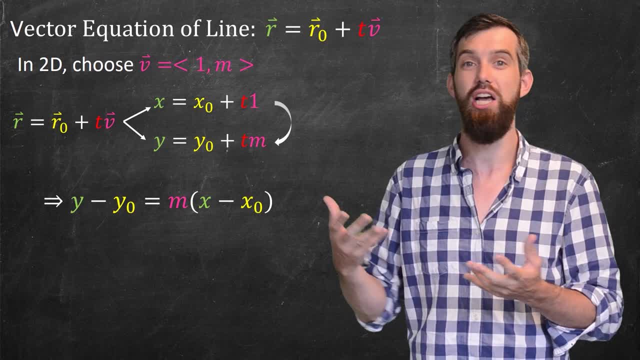 y minus y-naught is m x minus x-naught. So indeed, these two different ways of thinking about it, they are exactly the same.